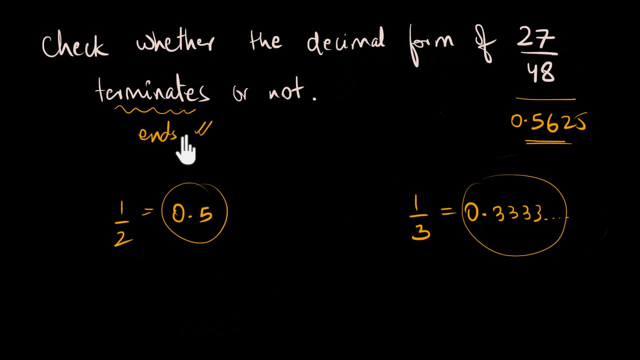 So you're looking for a way to solve this question without a calculator, And that's what we're going to do. But instead of giving away that method, what I would like us to do is together discover that method. So by the end of this video, we'll be able to look at any fraction, not just this one. 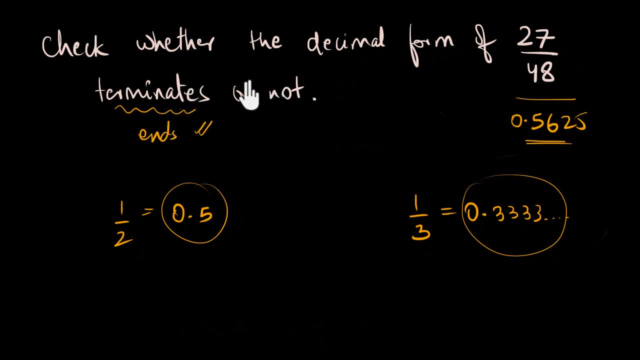 and talk about its decimal form, whether it terminates or not, And, more importantly, we'll have a very clear idea of why that method works. So let's get started. Let's actually try to find the decimal form of 27 by 48, whether it ends or does it look something like this: 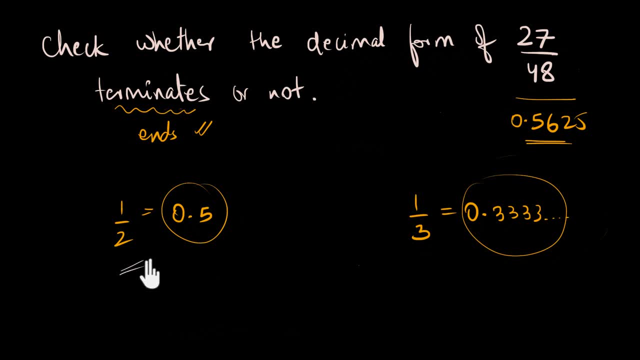 connection between fractions and decimals. What is it about these fractions that tell us whether the decimal form will end or will never end? To solve this mystery, we need a couple of more examples. Let me clean this board and start writing a few decimals and. 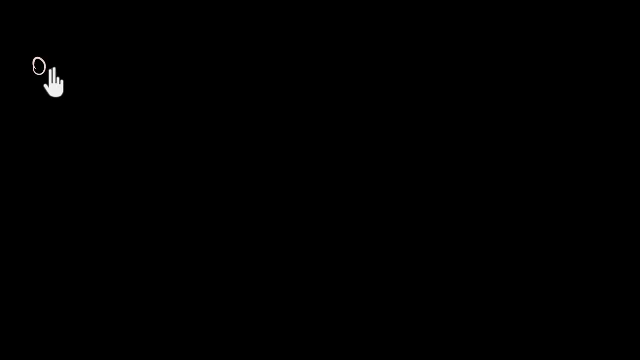 fractions. Let me first write a few decimals that end: 0.2 ends, 1.25 ends and 0.175.. All of these three end. I'm calling it decimals that end or they terminate. Okay, let me write a few more decimals, a few that don't end. I'll pick a few common ones. 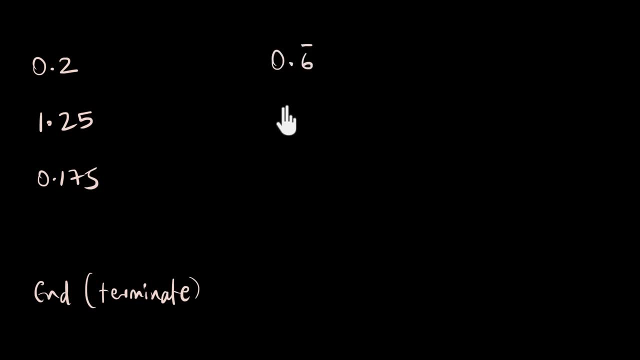 0.6 bar, 0.6, repeating. Then there's this 0.83 bar and here's one of my favorite: 0.142857.. All of this repeating These decimals don't end. I'm going to call it, don't end. They are non-terminating. 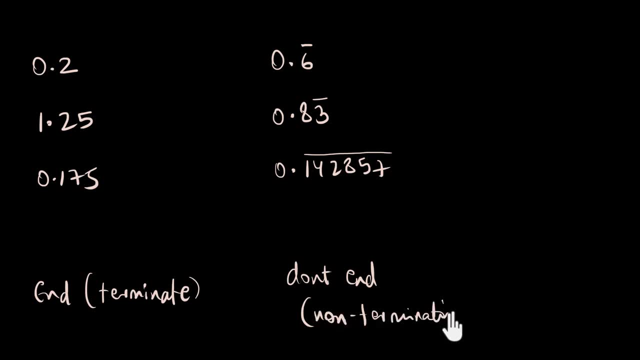 Non-terminating. Is there any other type of decimals? Well, there's one type which doesn't end but is also not repeating, like 0.125798 dot, dot, dot. So there's no clear pattern and it doesn't end. But I don't think we need to consider these type of decimals for this video, because we're 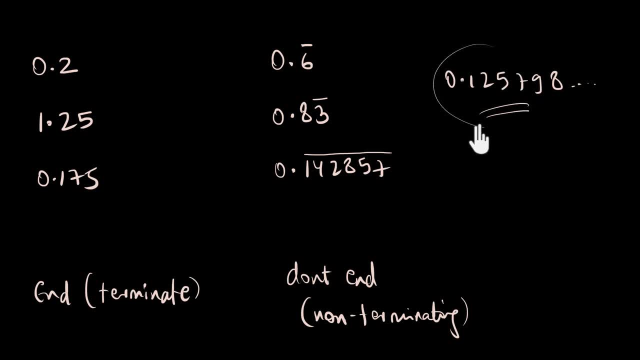 looking for a relation between fractions and decimals, and these decimals are not going to give us rational numbers. They're actually irrational numbers. So we don't get a fraction, We're not interested. Let's get rid of them and only look at these decimals. Okay, so now that we have these, 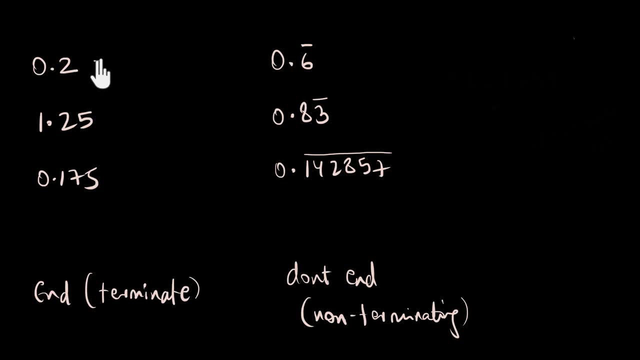 numbers in the decimal form. let's also write their fractional form. So 0.2 is actually 2 by 10.. 1.25 is 125 by 100.. 0.175 is 175 by 1000.. Here, because I don't really remember what these fractions are, 0.6 bar is actually 2. 3rd, 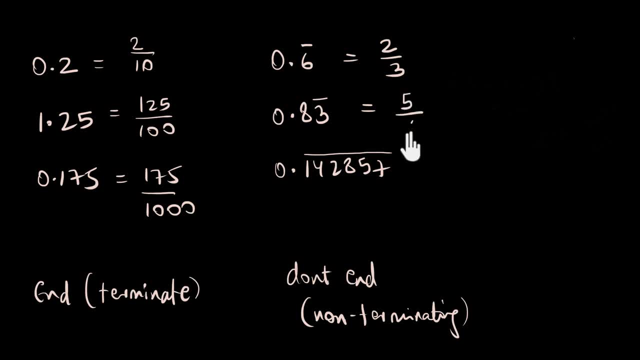 0.83 bar is. where is it? It's 5, 6th, 0.142857.. That's something that I remember. That's 1- 7th. So yeah, here are a few fractions which give us terminating decimals and a few fractions. 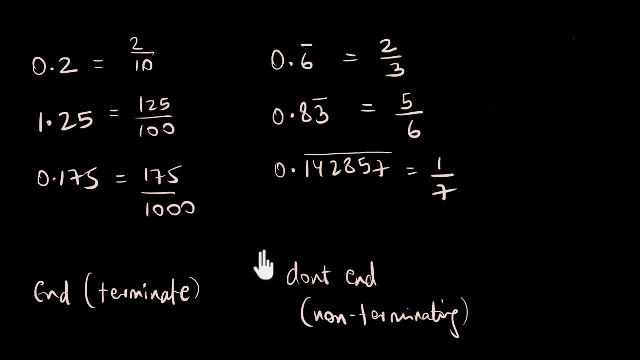 which give us non-terminating decimals. Can we see a pattern here? Do we have something special going on here, Something that's always giving us terminating decimals? Think about it. So did you see it? Here's the pattern, If you look at these fractions. 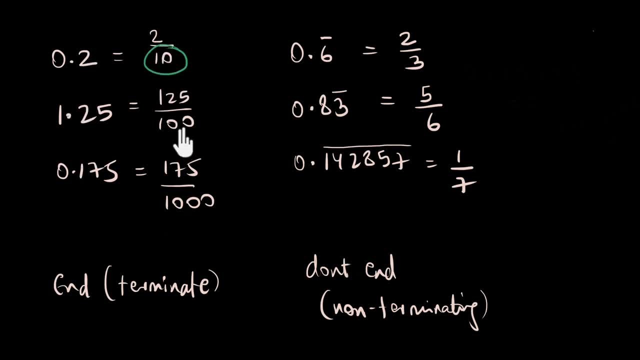 which give us decimals that end. these denominators are somewhat special. All of these denominators are multiples of 10.. No, wait, powers of 10.. It's the first power, second power and the third power, And you don't see that here, So maybe 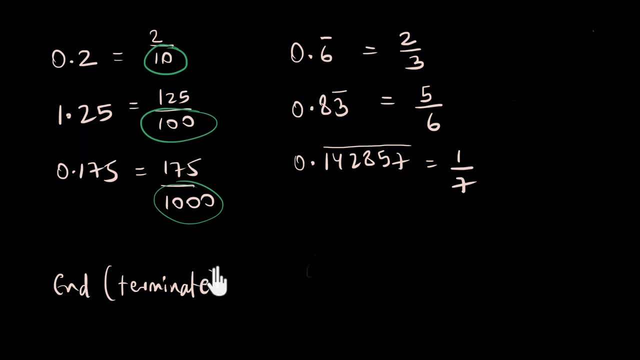 maybe for a fraction to give us a decimal that end, we need its denominator. I'm going to write dr here. Its denominator should be be a power of 10.. Power of 10.. Now, this does make sense, but let's. 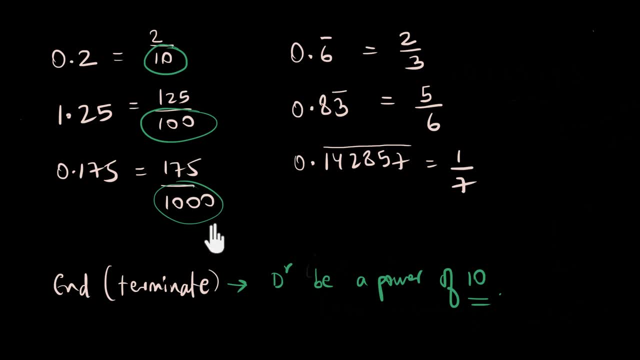 be really sure about this. Is there no other fraction that does the job? Hmm, Well, I can think of a few. We started this video with the fraction half. Now half gives the decimal 0.5, which is terminating, And this is not a power of 10. So clearly there's something else going on, And here's. 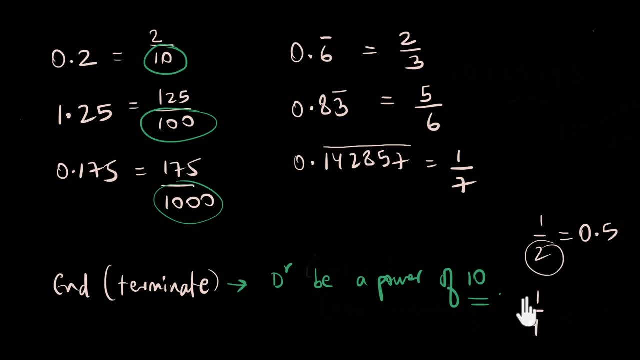 one more number that breaks the rule 1 by 4, which is a quarter, This gives us 0.25.. Even that's terminating, And this is not a power of 10.. Hmm, I think we jumped to this conclusion a bit too fast, because even here I can see some. 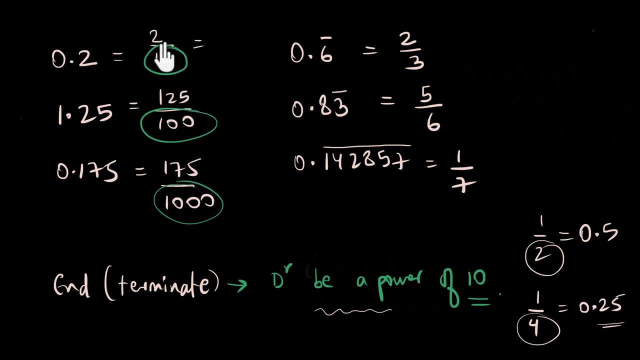 nonpowers of 10.. If I simplify these fractions, I'll get: this is 1 by 5.. This is 5 by 4.. And this is: if I cancel 25 out, I'll get 7 by 40.. So I can see these numbers. 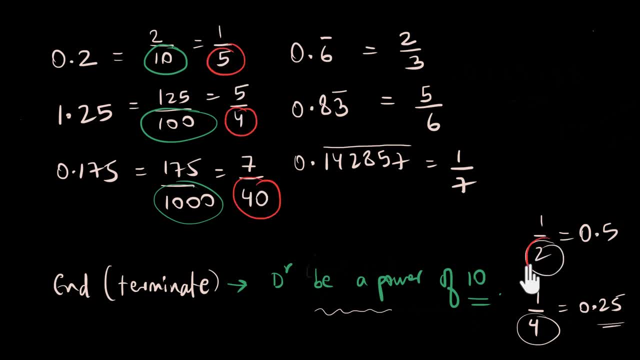 5,, 4,, 40, and even 2.. I can see these numbers popping up, and and none of these numbers are powers of 10.. So now, what do we do? What's so special about these denominators that are giving? 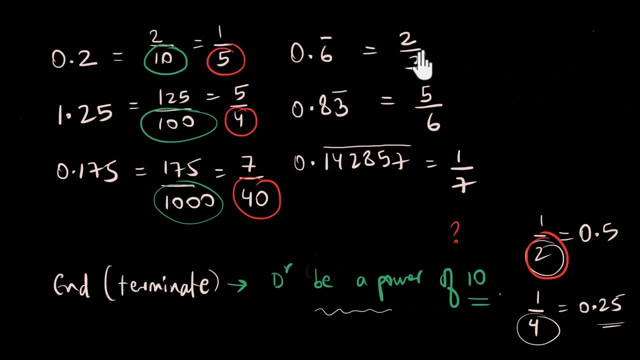 us terminating decimals. What do these numbers have that these numbers don't? 3,, 6 and 7.. Pause for a moment and see if you can figure it out yourself, Okay, So here's what's going on. Let me clean this up first. 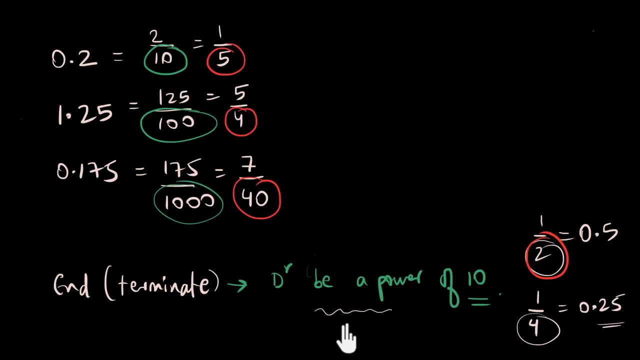 So now this is what's going on. Let me clean this up first. here's what's going on. We still need powers of 10 in the denominator to get these decimals that end, but we don't always need to start with these powers of 10.. We can start with some other numbers. 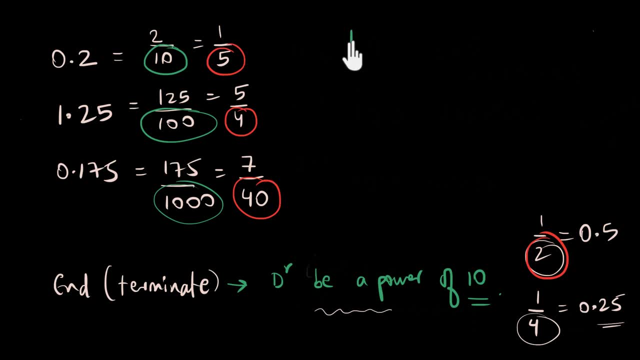 like these, And here's why they work. If you look at 10, that's made up of a, 2 and a 5.. And all higher powers of 10 are also made up of 2s and 5s. 100 is made up of 2, 2s and 2- 5s. 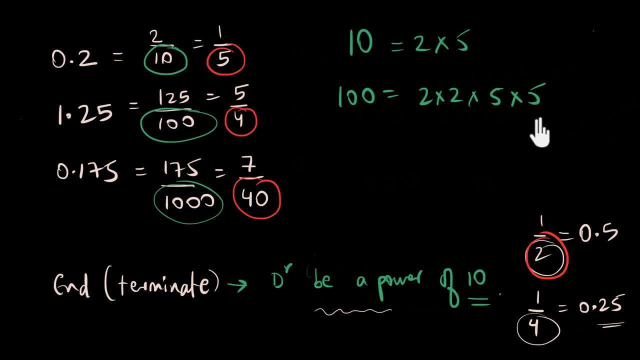 Similarly, 1000 will be made up of 3 2s and 3 5s, So you can start with 10, but you can also start with a 5.. If you have a 5 in the denominator, simply multiply numerator and denominator by 2. 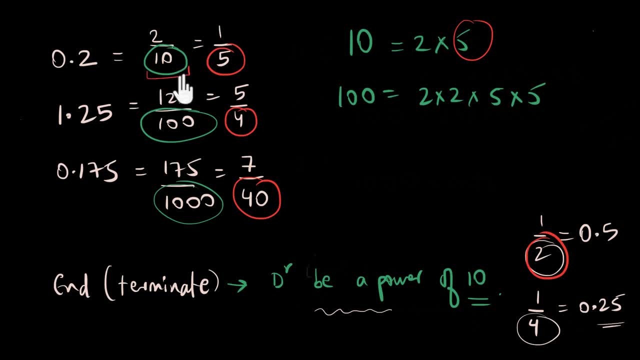 to get 2 by 10, and there you have it: a 10 in the denominator. That will give you a terminating decimal, And this is what's happening for all of these numbers. If you look at 4,, that's actually. 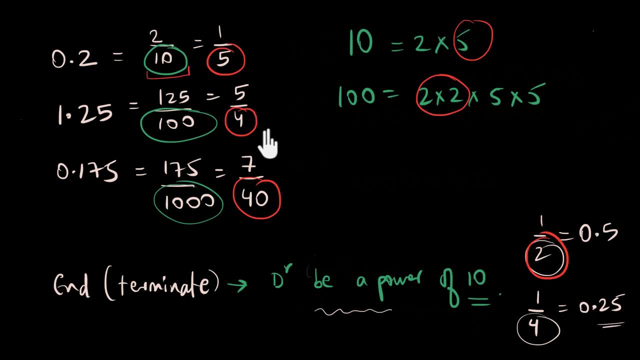 2 times 2.. To make it a power of 10, you multiply this by 25.. Now let's look at 40.. 40 is made up of: if I factorize 40, that's made up of a 2 and a 2 and a 2 and a 5.. 8 times 5 is 40. To make this: 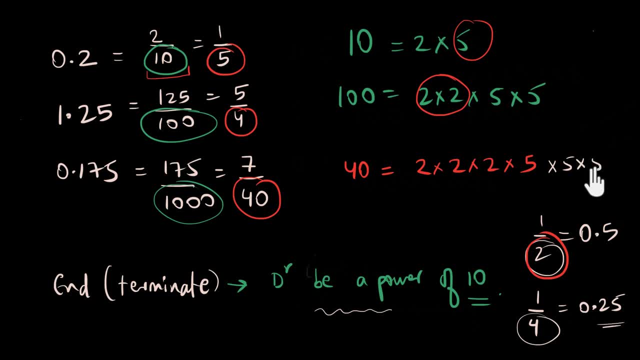 a power of 10,. we'll multiply this by 5 times 5,, which is 25.. This will give us 1000.. And that's exactly what's going on here, And this also explains why the other fractions were not working. 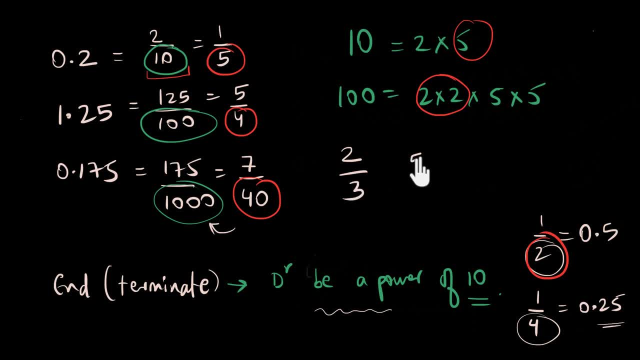 We now know why 2 by 3 was not working and 5 by 6 was not working and 1 by 7 was not working. For all three denominators- 3, 6, and 7, we have numbers that will never give us 10.. There is no integer that you can multiply 3 with. 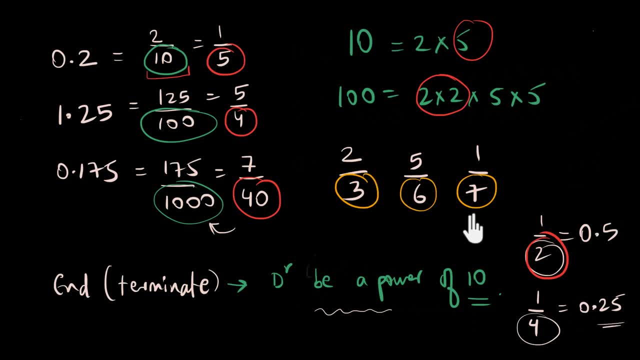 to get 10 or a power of 10.. And that's the problem with these two as well. Okay, I think we've figured it out. Now let's summarize: If we want a terminating decimal, if we want a decimal that ends, we need to start with a fraction that has a power of 10 in the denominator. But if you're not, 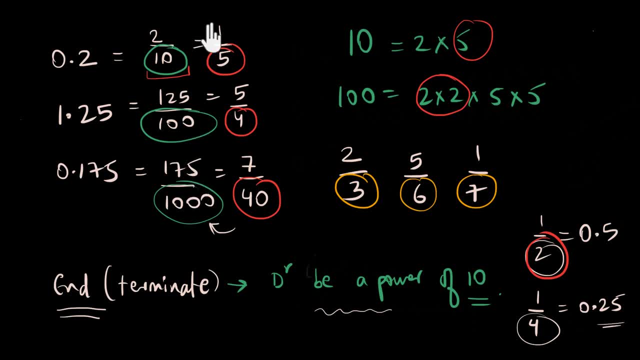 that lucky. if we don't have a power of 10, then at least we should start with a number that has only 2s and 5s in the denominator, And that's the problem with these two as well. Now let's summarize. 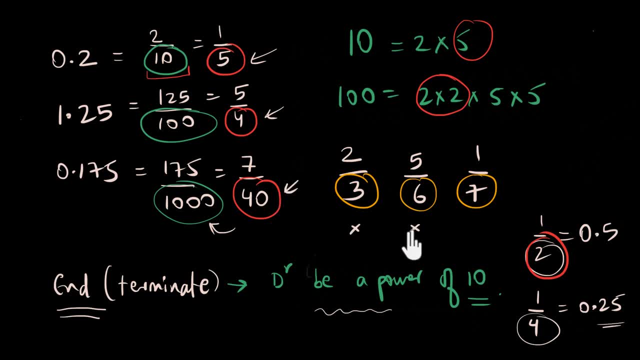 If we start with anything else, then we're not going to get a terminating decimal. Isn't that amazing? Just by looking at these denominators, we can figure out whether the decimal is going to end or not end. I'm excited to try a few more problems. Let's get this out. 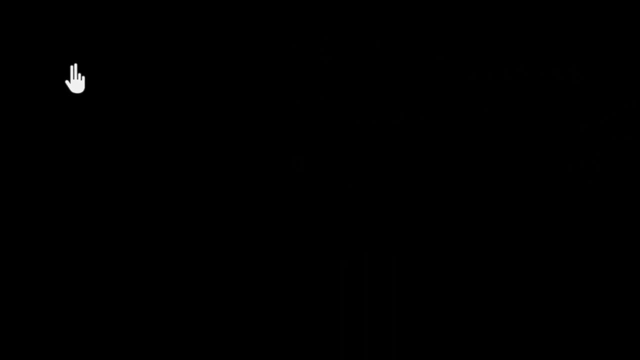 And this time we're not going to use a calculator. So let me write down a few fractions: 13 by 12, and let's add one more, 29 by 35, and one more 21 by 30.. Pause the video and check whether these fractions are going to give us. 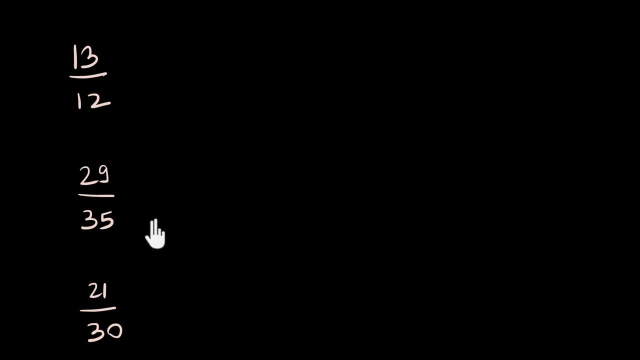 terminating decimals or non-terminating decimals. Okay, so let's do this together. If you look at the denominator, we have 12.. And 12 is made up of a 2 and a 2 and a 3.. 2s are fine, but this 3 is going to be a problem, So this is not going to give us. 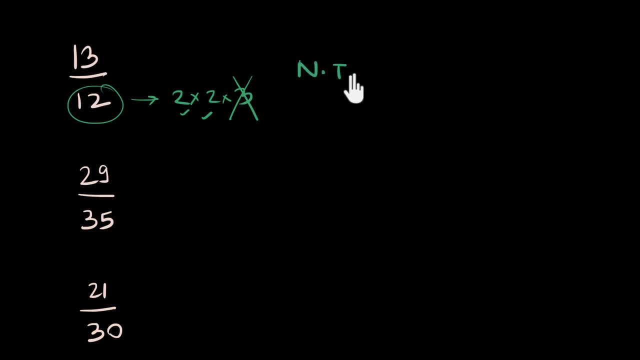 a terminating decimal. This is going to give us a non-terminating decimal. What about 29 by 30? 35.. Well, 35 is made up of a 5 and a 7.. 5 is fine, but 7 is a problem. 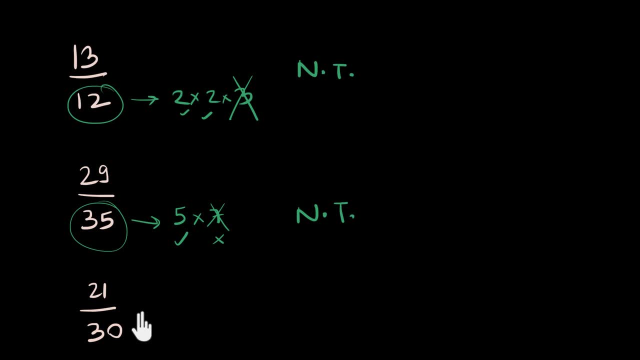 7 is a problem. so a non-terminating decimal. And don't you remember 30?? If you look at 30, it's made up of a 2 and a 5 and a 3.. 2 is fine, 5 is fine, but 3 is a problem. 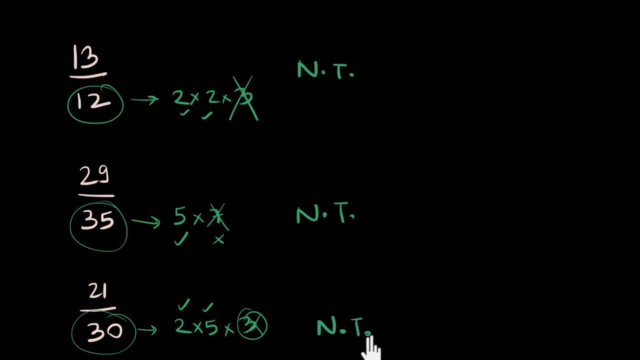 So this is also going to give us a non-terminating decimal. Now let's check our answers using a calculator: 30 by 12 is actually 0.0134133333333333333333333. re 3 is repeating. so yeah, that's going to give us a non-terminating. 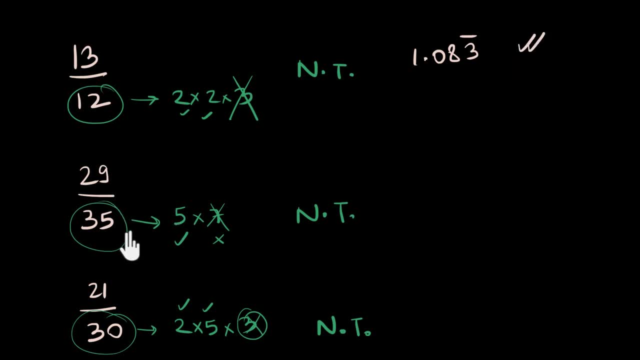 decimal, So we were right. 29 by 35 is actually 0.8285714.. Okay, that's really a long one, but it's also repeating, and this is not going to end. It's a non-terminating decimal, So we were right. 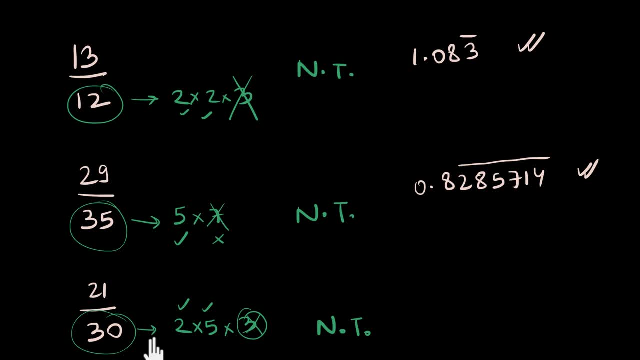 And the third one is 21 by 20.. That's actually 1.0823443333333333333, 0.7.. Okay, hold on, Something's wrong. This was supposed to be a non-terminant decimal, but 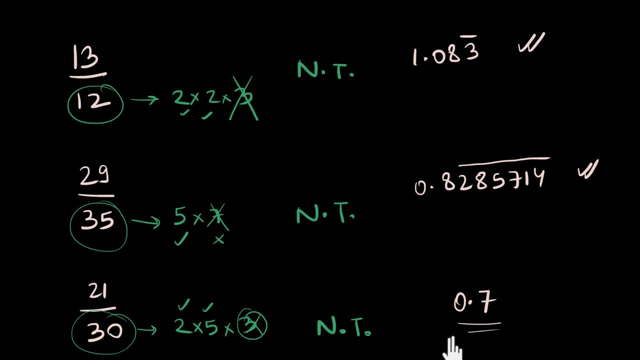 why did it end? Try to pause the video and see if you can figure out what's going on here. Okay, are you ready? Did you see it? 21 by 30.. We had a 2 and a 5 and a 3, which was a problem. 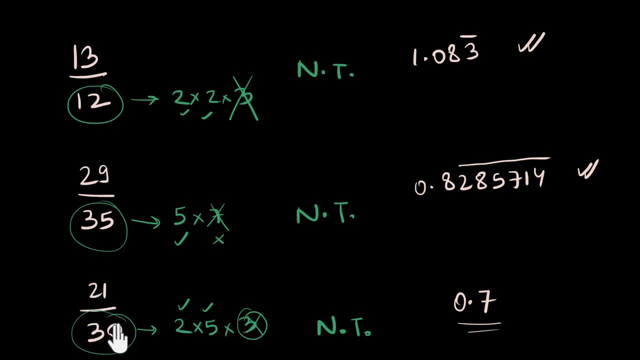 but all this while we were only looking at the denominator. If I also look at the numerator 21,. that's made up of a 3 and a 7. Surprisingly, this 3, which was a problem in the denominator- 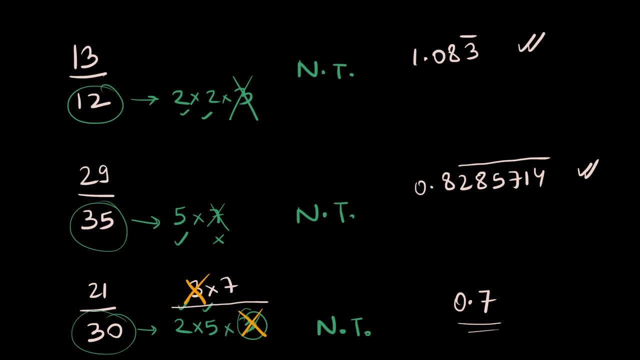 actually gets cancelled out. So my fraction becomes- I'm going to get rid of nt- my fraction becomes 7 upon 2 times 5, which is 10, and 10 will always give us a terminating decimal. So we should still check for these 2s and 5s in the denominator, but only after we have the 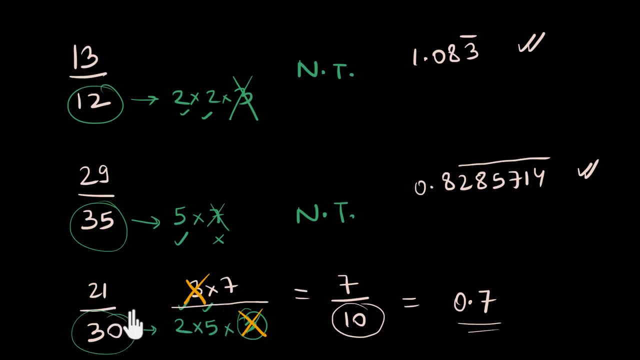 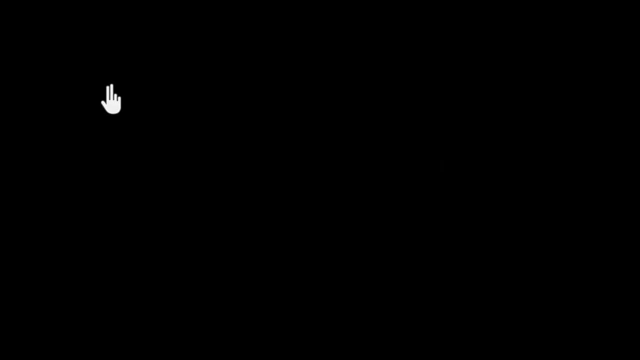 fraction written in the simplifier, In the simplified form. we should make sure that everything that's a problem actually gets cancelled out first. Okay, now let's really summarize. Let's do that using the first question that we started with. We had 27 by 48, and we know that this is going to be 0.5625,, but suppose we 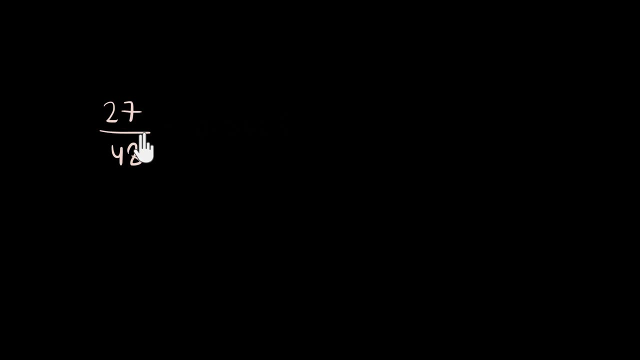 don't have the calculator and we want to know whether this fraction terminates or not in the decimal form. What do we do? So the first thing that we do is we prime factorize. We see that that's made up of a 2 and a 2 and a 2 and a 2, that's 16, and one more 3. That's 3.. And the 2s are: